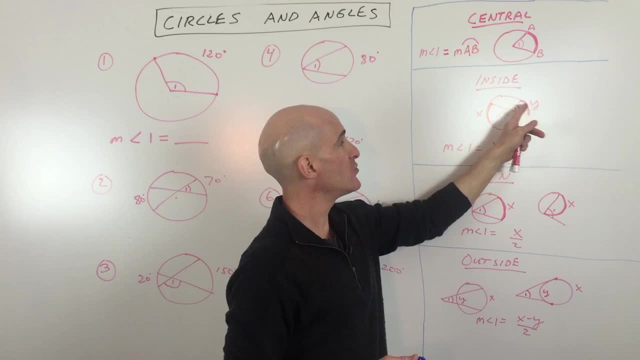 they're intersecting inside the circle, and what you want to do is you want to actually average these two intercepted arcs. you want to add arc x and arc y together, divide by two, so it's like taking an average, and you're going to get the measure of angle one. now notice that this angle 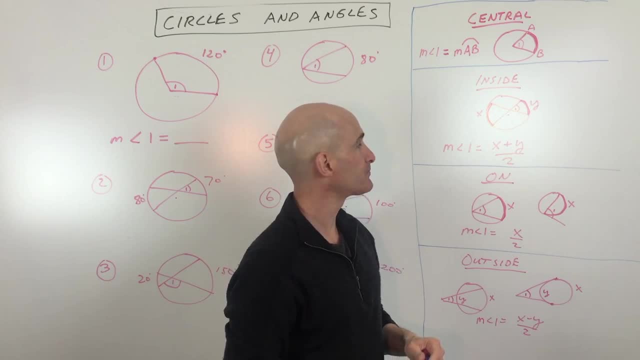 and this angle are vertical angles, so they're going to be the same, they're going to be congruent. if you want to solve for this angle here, though, you would either need to know these two arcs, okay, or if you know this angle, you can subtract from 180, since 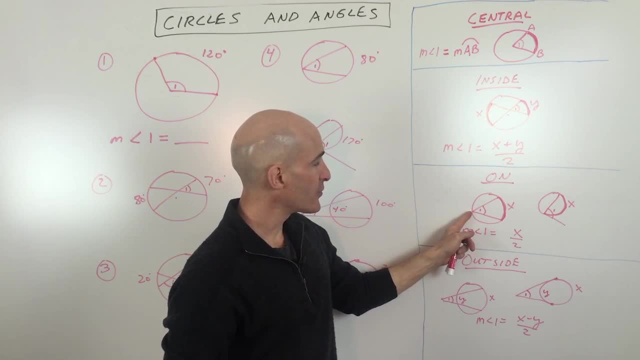 those are a linear pair. okay, this one. here you can see the vertex of the angle is on the circle. okay, see the vertex, the hinge right of the angle, it's right on the circle and that angle here is called an inscribed angle. okay, it's inside the circle, but it's going to be half of the 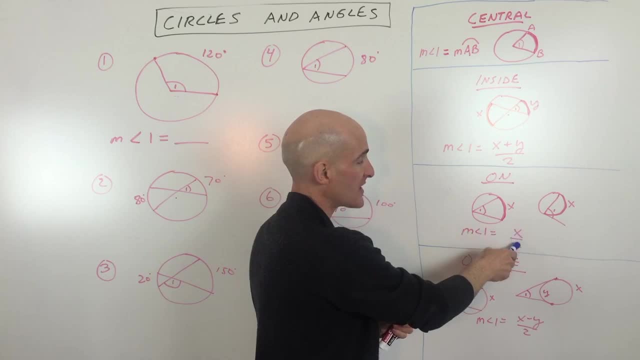 intercepted arc. so if this is x, the measure of angle one is half of that. over here we have a chord. okay, this is the chord and this is the tangent, but again you can see the vertex is right on the circle and the measure of the angle one is going. 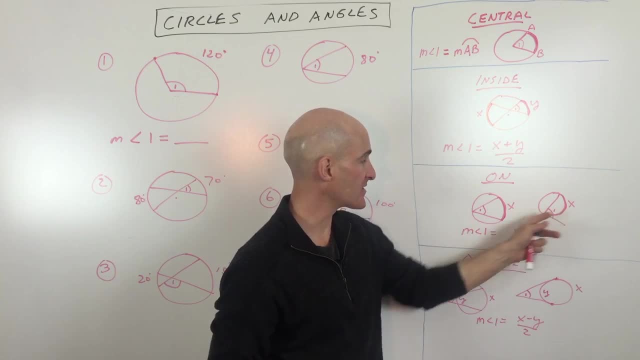 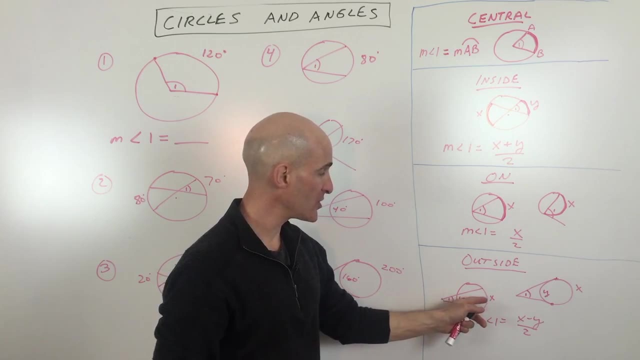 to be half of that intercepted arc. in this case i'm just calling it x. so the same formula. and then the last one. we have the outside. so the vertex of the angle is outside the circle and what you're doing is you're actually subtracting. it's the larger arc minus the smaller arc, divided by two. 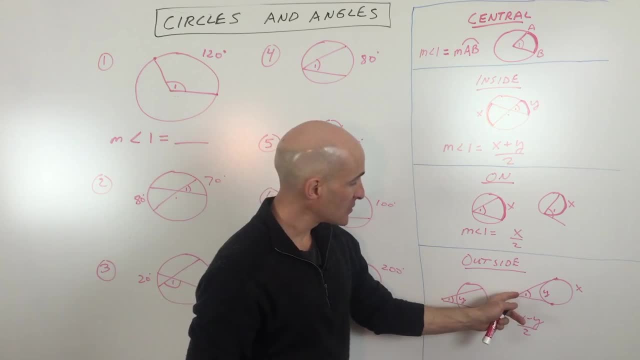 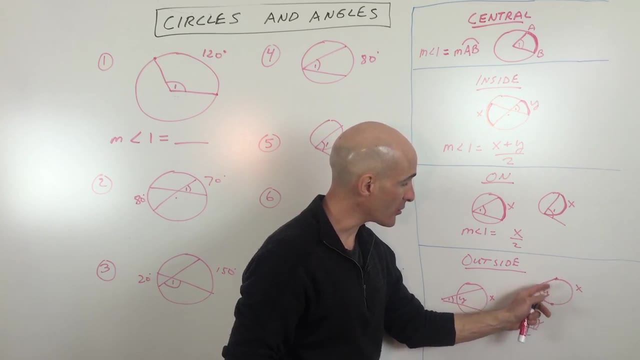 so this arc minus this arc divided by two, this one over here. we have two tangents, but again you can see the vertex of the angle one is outside the circle. you're going to take this larger arc or the one that's further away from angle one minus the smaller one, which 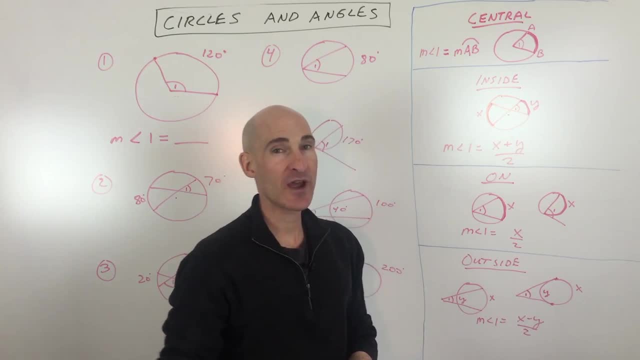 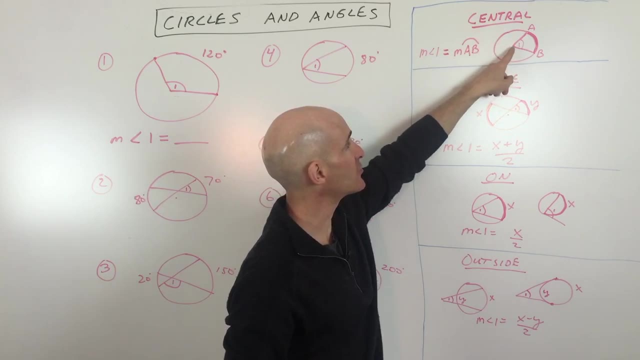 is actually closer to angle one, and then divide by two. so what i've tried to do for you here and for myself, just to make memorizing the formulas easier- is to group them so you can think about the central angle. okay, half of the intercepted arc, no, okay, i'm sorry. 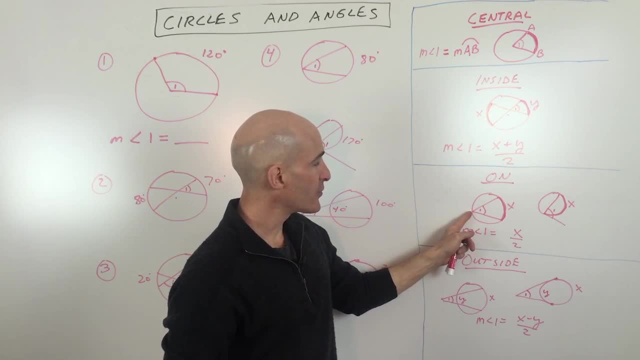 those are a linear pair. okay, this one. here you can see the vertex of the angle is on the circle. okay, see the vertex, the hinge right of the angle, it's right on the circle and that angle here is called an inscribed angle. okay, it's inside the circle, but it's going to be half of the 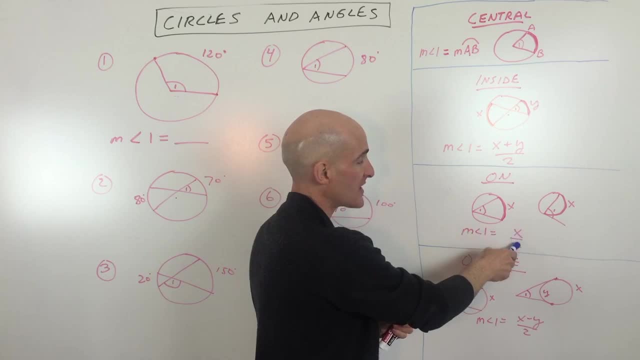 intercepted arc. so if this is x, the measure of angle one is half of that. over here we have a chord. okay, this is the chord and this is the tangent, but again you can see the vertex is right on the circle and the measure of the angle one is going. 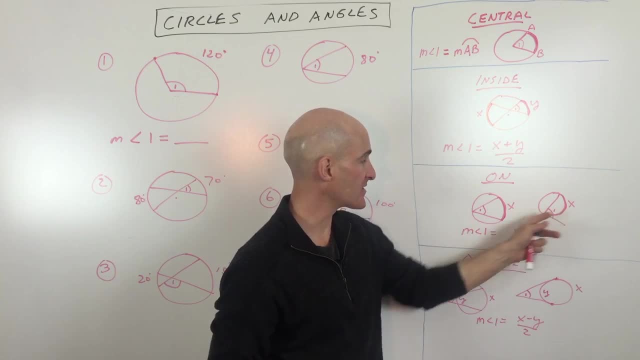 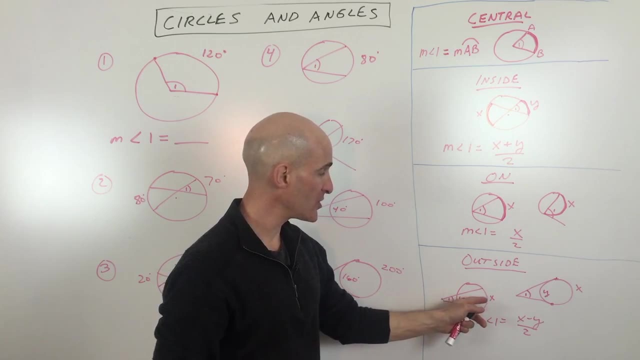 to be half of that intercepted arc. in this case i'm just calling it x. so the same formula. and then the last one. we have the outside. so the vertex of the angle is outside the circle and what you're doing is you're actually subtracting. it's the larger arc minus the smaller arc, divided by two. 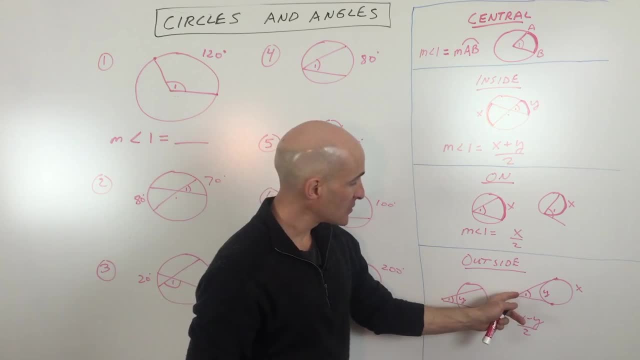 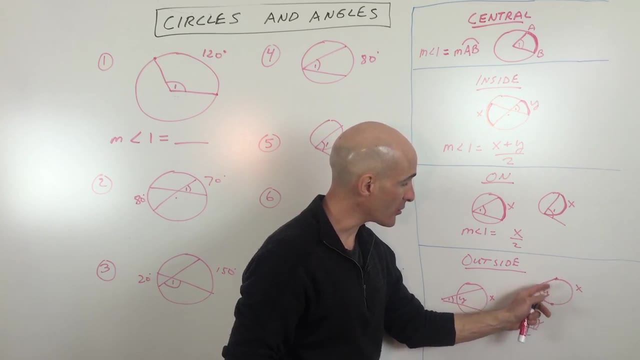 so this arc minus this arc divided by two, this one over here. we have two tangents, but again you can see the vertex of the angle one is outside the circle. you're going to take this larger arc or the one that's further away from angle one minus the smaller one, which 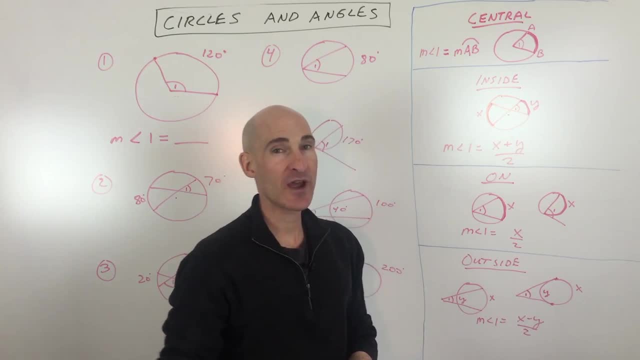 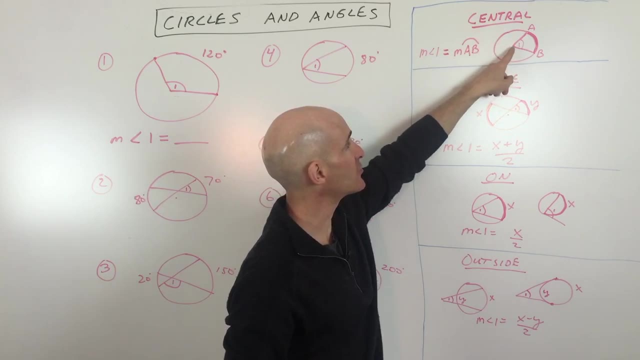 is actually closer to angle one, and then divide by two. so what i've tried to do for you here and for myself, just to make memorizing the formulas easier- is to group them so you can think about the central angle. okay, half of the intercepted arc, no, okay, i'm sorry. 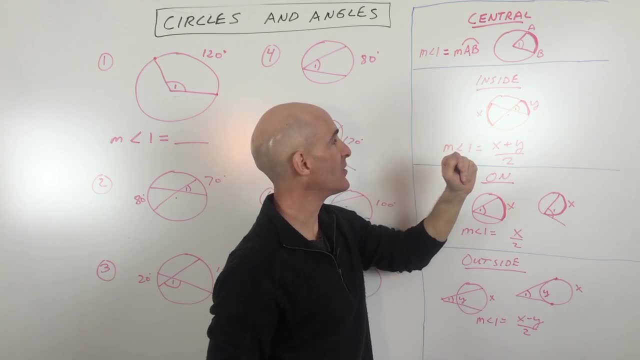 central angle it's the same as the intercepted arc inside. okay, it's an average of the two arcs. you're adding up and dividing by two. on the circle you're taking half of the intercepted arc and then outside the circle you're subtracting and dividing by two. so if you can look at where, 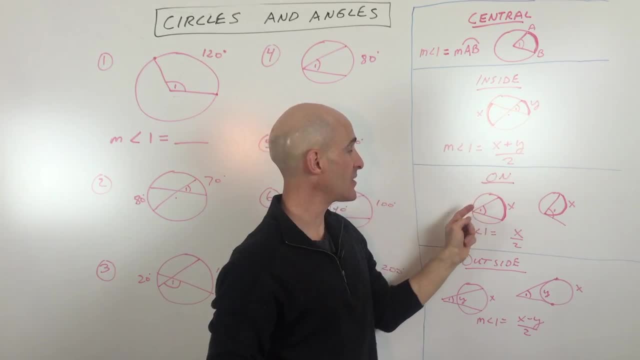 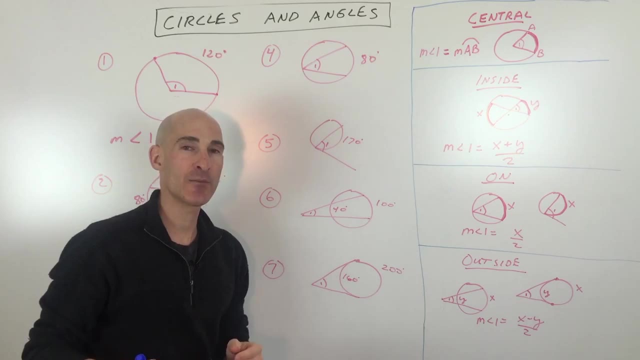 that vertex is located at the center inside, but not at the center on the circle or outside the circle. that'll help you to figure out which formula to use. we're going to go through some examples and you've got a couple options here. one option is you might want to look at these pause. 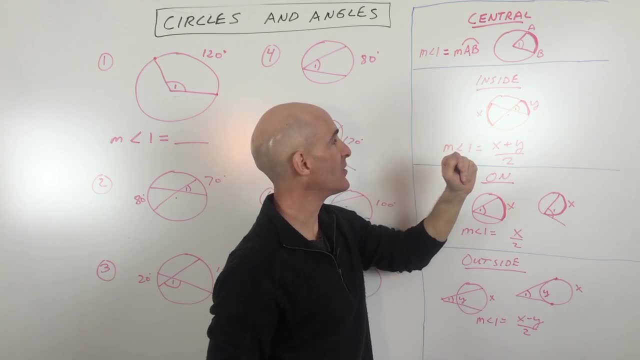 central angle it's the same as the intercepted arc inside. okay, it's an average of the two arcs. you're adding up and dividing by two. on the circle you're taking half of the intercepted arc and then outside the circle you're subtracting and dividing by two. so if you can look at where, 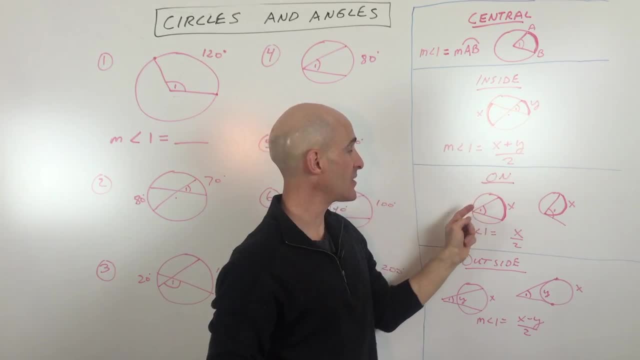 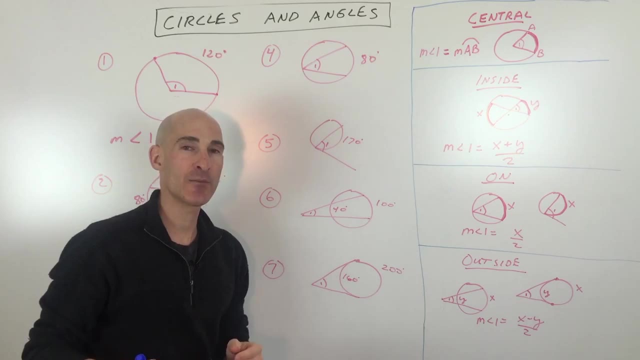 that vertex is located at the center inside, but not at the center on the circle or outside the circle. that'll help you to figure out which formula to use. we're going to go through some examples and you've got a couple options here. one option is you might want to look at these pause. 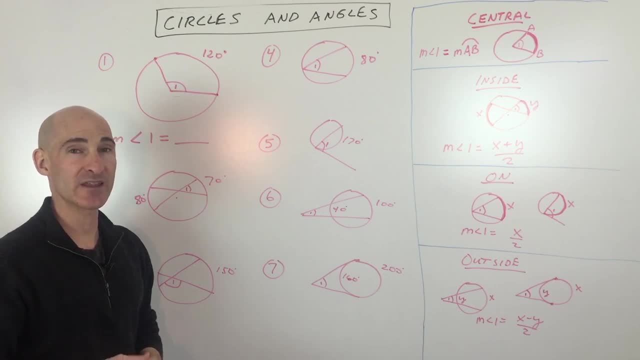 the video, see if you can solve them yourself, and then go ahead and replay it and then see if you've got them right or if you just want to use those different options. you can go ahead and want to follow along. that's fine too. so let's see if we can go through them. so this one here. 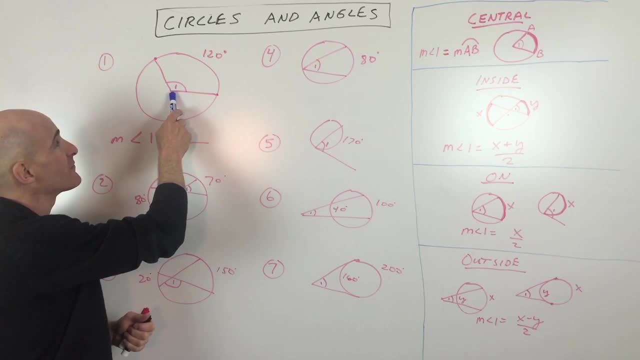 what do we do to find angle one? well, since the vertex is right at the center, this angle is going to have the same measurement as the intercepted arc, okay, which is 120. so this one angle one is just going to be 120 degrees. okay, that one was pretty easy. okay, this one over here. now you can. 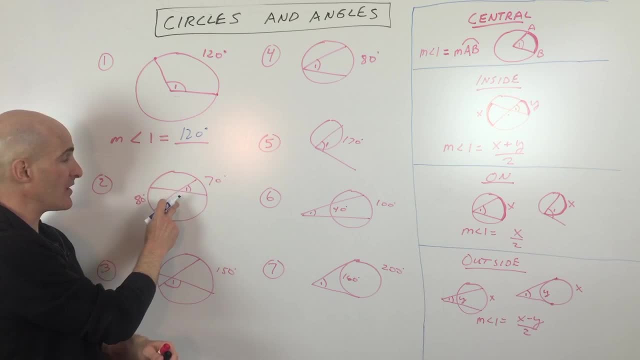 see that the vertex of angle one. it's inside the circle, okay, but it's not at the center. so here, what we're going to do is we're going to add up the two intercepted arcs- 80 plus 70, okay, 80 plus 70- and we're going to divide that by 2, so that's 150 divided by 2, 75 degrees. okay with me so far. 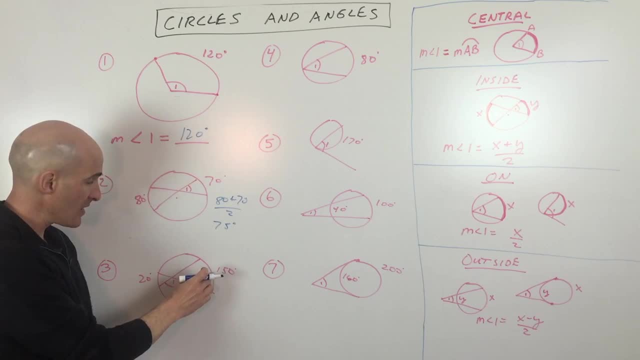 now this one over here is pretty much the same setup. okay, you can see the vertex of the angle. angle one is inside the circle. we're going to add up the two intercepted arcs. we're going to divide by 2. okay, so that's 170 divided by 2 is 85. but you can see that's this angle here. so if you 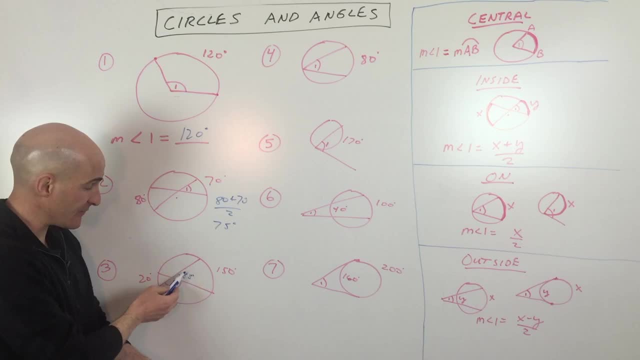 want to solve for angle one, we actually have to take 180 minus 85, since these form a linear pair, so angle one here is actually going to be 95 degrees. okay, if we knew these two arcs, we could add those up and divide by two, but in this case they just gave us these two, so we worked with what? 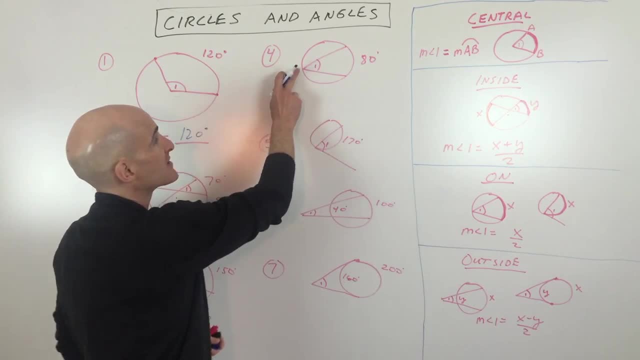 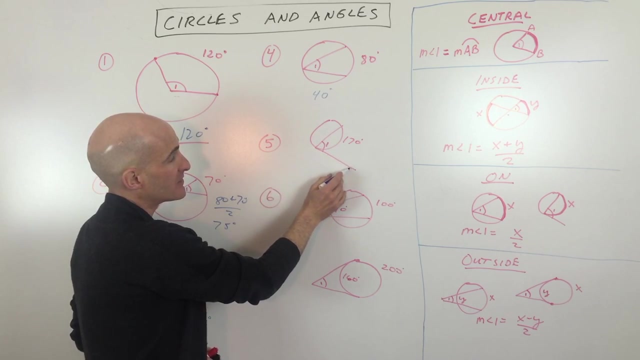 we had, okay, number four: notice that the vertex is on the circle. this is called an inscribed angle, okay, and this is going to be half of the intercepted arc, so half of 80 degrees. so this is just going to be 40 degrees, this one. here also, the vertex is on the circle. okay, you have a tangent. 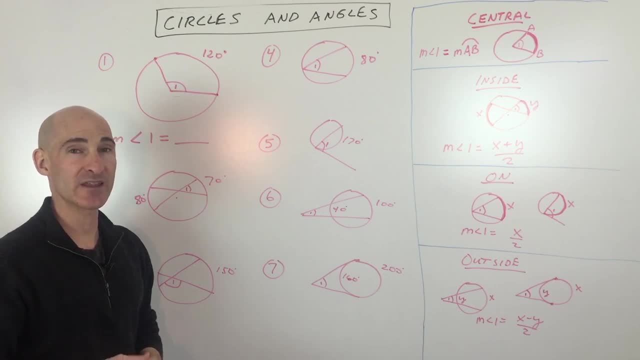 the video, see if you can solve them yourself, and then go ahead and replay it and then see if you've got them right or if you just want to go back and look at your formula and solve it yourself. want to follow along? that's fine too. so let's see if we can go through them. so this one here. 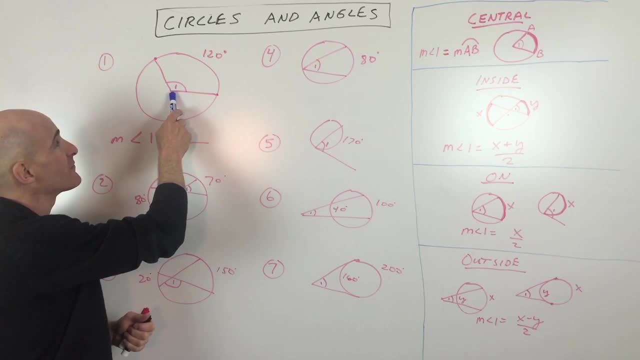 what do we do to find angle one? well, since the vertex is right at the center, this angle is going to have the same measurement as the intercepted arc, okay, which is 120. so this one angle one is just going to be 120 degrees. okay, that one was pretty easy. okay, this one over here. now you can. 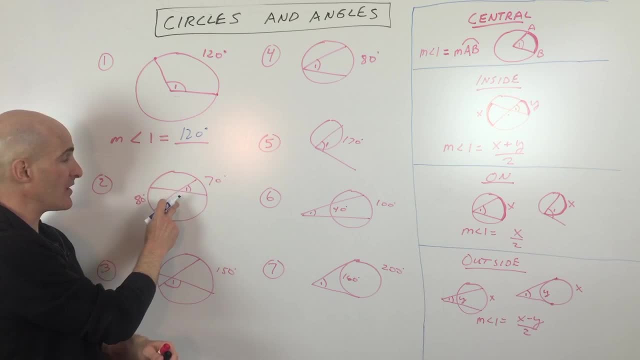 see that the vertex of angle one. it's inside the circle, okay, but it's not at the center. so here, what we're going to do is we're going to add up the two intercepted arcs- 80 plus 70, okay, 80 plus 70- and we're going to divide that by two. so that's 150 divided by two, 75 degrees. okay with me so far. 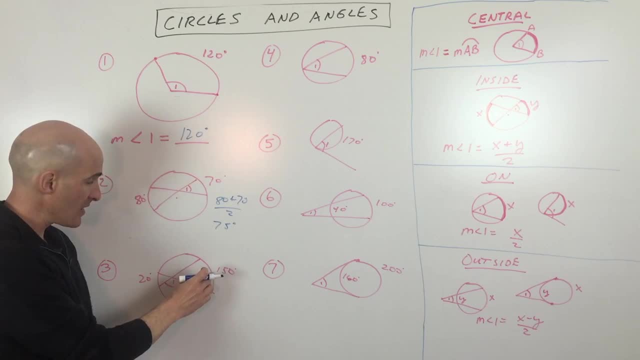 now this one over here is pretty much the same setup. okay, you can see the vertex of the angle. angle one is inside the circle. we're going to add up the two intercepted arcs. we're going to divide by two. okay, so that's 170 divided by two is 85. but you can see that's this angle here. so if you 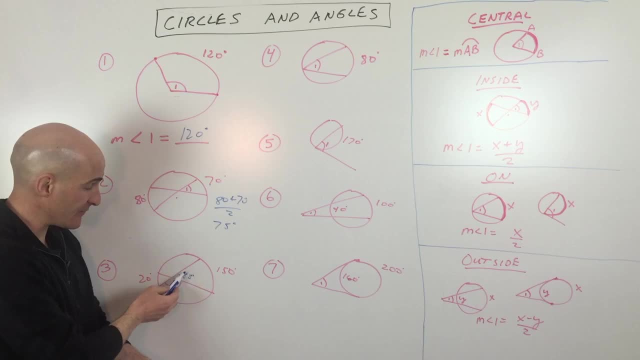 want to solve for angle one, we actually have to take 180 minus 85, since these form a linear pair, so angle one here is actually going to be 95 degrees. okay, if we knew these two arcs, we could add those up and divide by two, but in this case they just gave us these two, so we worked with 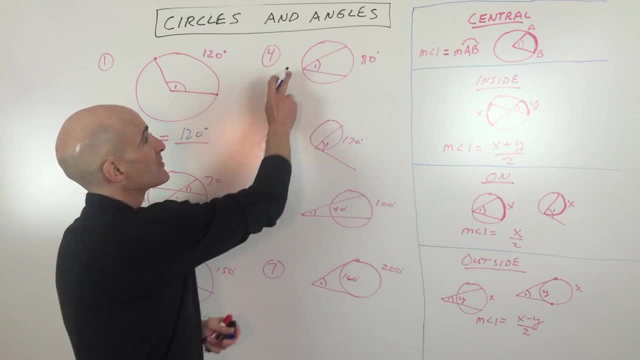 what we had. okay. number four: notice that the vertex is on the circle. this is called an inscribed angle, okay, and this is going to be half of the intercepted arc, so half of 80 degrees. so this is just going to be 40 degrees, this one. 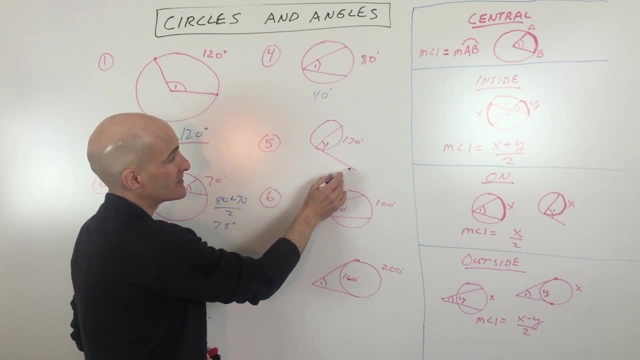 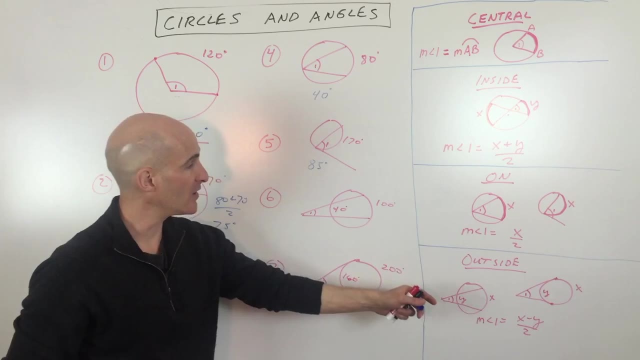 here also, the vertex is on the circle. okay, you have a tangent and a chord, so it's gonna be half of the intercepted arc, half of 170, which is 85. okay, we're just using this formula over here, okay, and then over here. now you can see the. 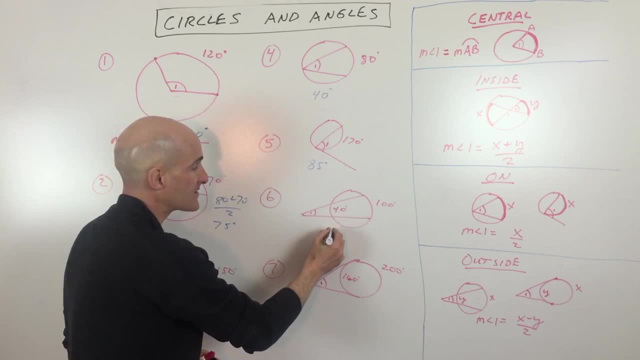 vertex is outside the circle. we're gonna be taking the larger arc minus the smaller arc divided by 2, so that's 60 divided by 2, which is 30 degrees. okay, so angle 1 is 30 and the last one here they give us, this is 200, this is 160. 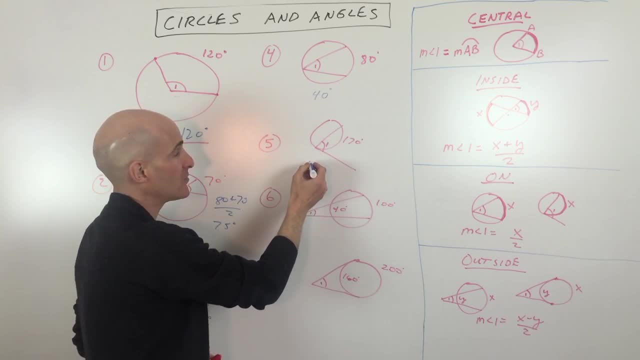 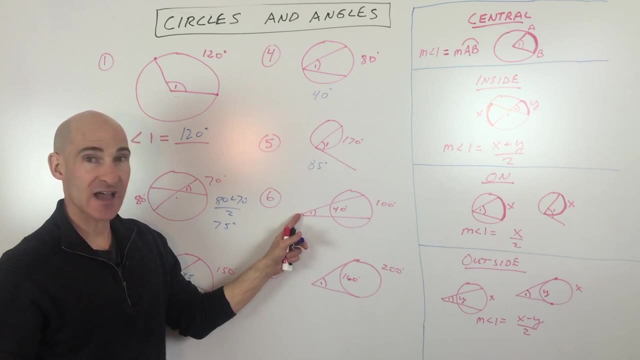 in a chord. so it's going to be half of the intercepted arc. 1x1 70, which is 85. okay, we're just using this formula over here, okay, and then over here, and now you can see the vertex is outside the circle. we're going to be taking the larger arc minus the smaller arc divided by two. 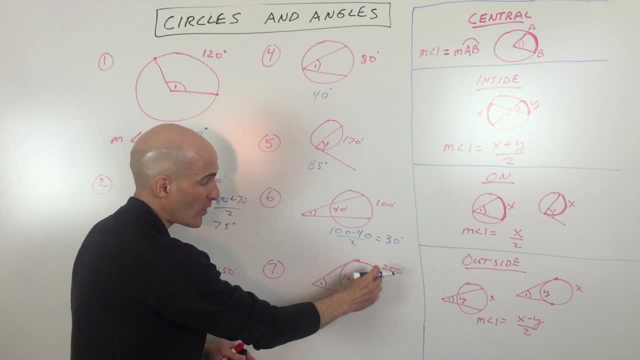 okay, so sometimes they won't give you this 160 degree value, but you want to realize that in a circle all the arcs are going to add up to 360 degrees. that's the arc sum formula. okay, and so we have 200 degrees minus 160 degrees.